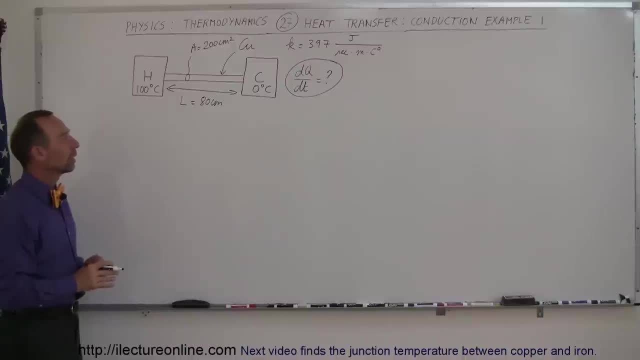 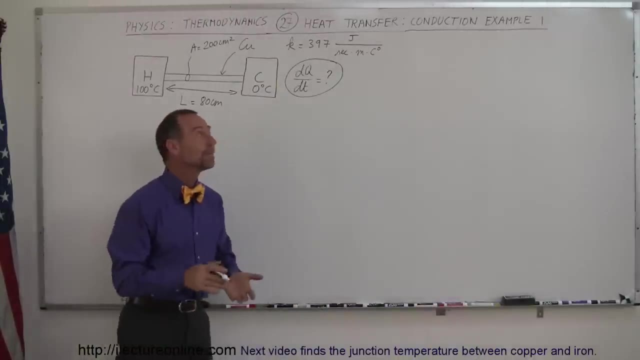 Let's assume that we ignore any radiation effects. The conductivity constant for copper is 397 joules per second per meter, per degree centigrade or per centigrade degree, And what we're trying to find is the amount of heat transferred across that interface, the dqdt. 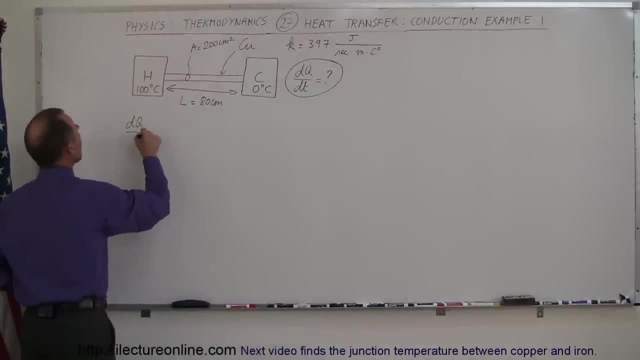 And the equation for the dqdt- dqdt, that just simply means the amount of heat transferred per unit time- per unit time typically is per second- is equal to 90. So the bigger k the conductivity constant, the greater the conductivity constant, the greater the propensity for the material to conduct heat. 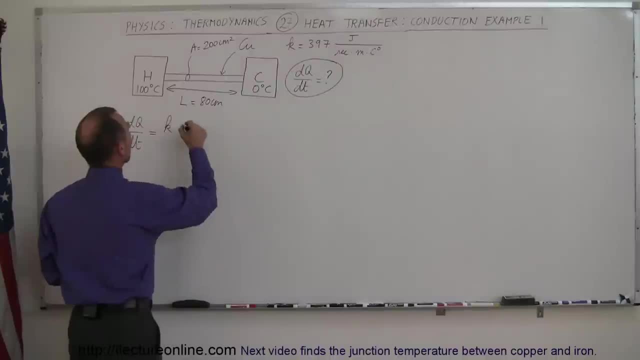 So the bigger k, the more heat will transfer The cross-sectional area, the more the bigger the path is. of course, the better the heat will transfer And the difference in the temperature between the hot and the cold reservoir The bigger the difference. the faster heat will travel down that path. 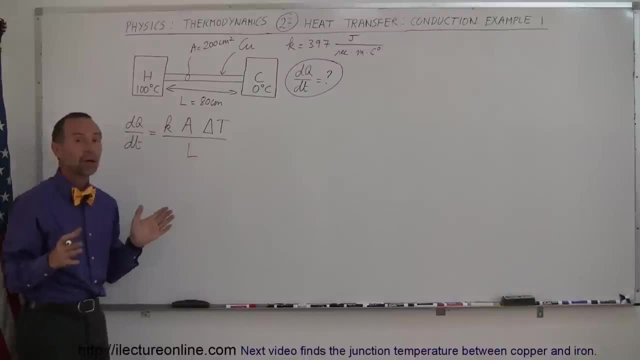 And then we have to divide that by the length, because the longer the path, the longer the path, The less heat will transfer. So a little path will transfer much quicker, A longer path, the heat will travel a lot slower. And there's a good reason for that, because, think about it. 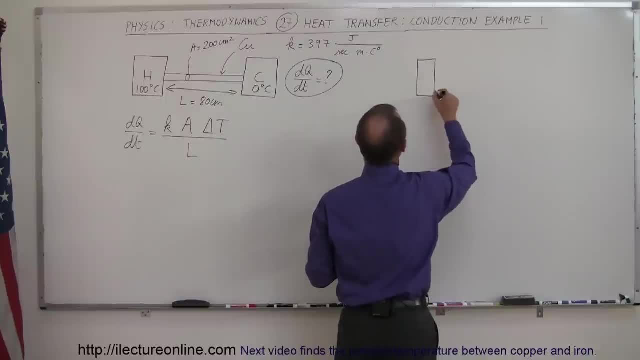 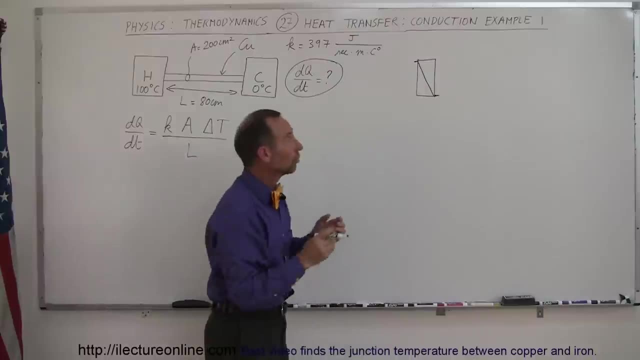 If the path is very short and the temperature on the hot side is over here and on the cold side is over there, we have what we call a very steep temperature gradient. The temperature difference across that interface changes very quickly, which would cause a lot more heat to transfer. 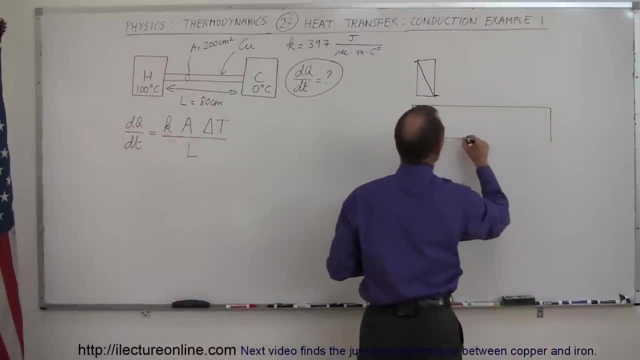 If the path is much longer like so, and we have the temperature like this on one side and like this on the other side, you can see that the temperature gradient is much more gradual and therefore a lot less heat will transfer from the hot to the cold. 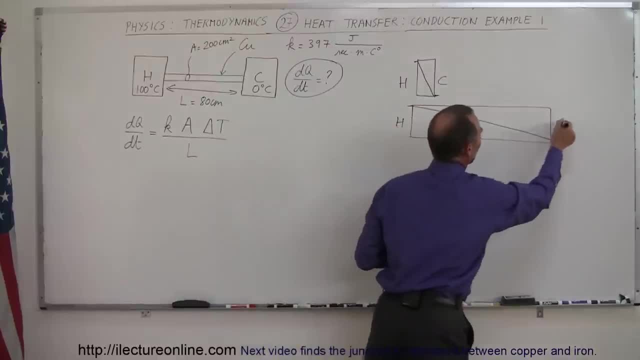 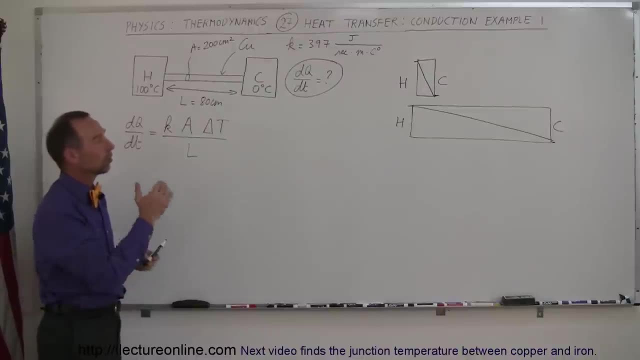 So again, this would be hot, this is cold, this is hot, this is cold. So you can see visually here that the longer the path, the slower or the smaller the temperature gradient and the slower heat will transfer across that path. 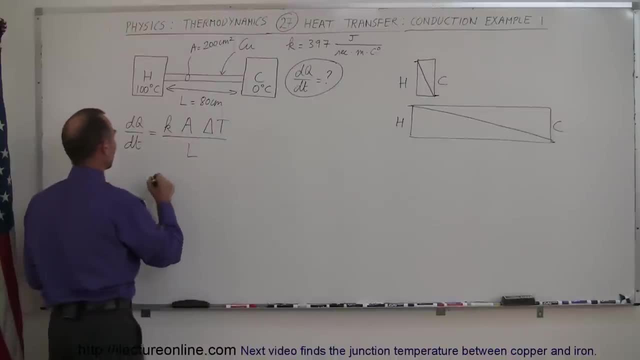 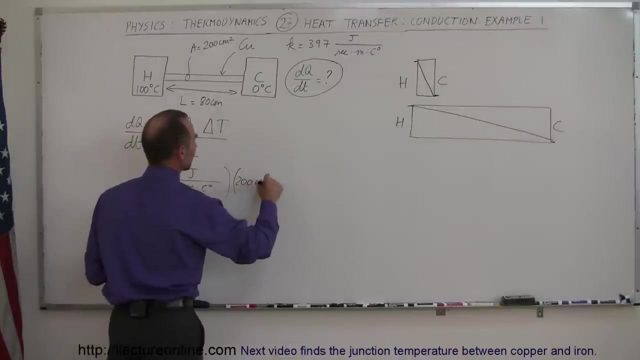 Okay, here's the equation. let's plug in the numbers that we have. So for K, we have 397 joules per second, times meters, times centigrade degrees, The cross-sectional area, which is 200 square centimeters, and then of course we have to convert that to square meters because we want to use standard units here. 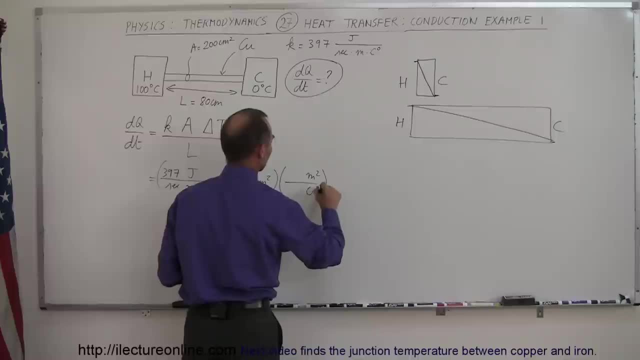 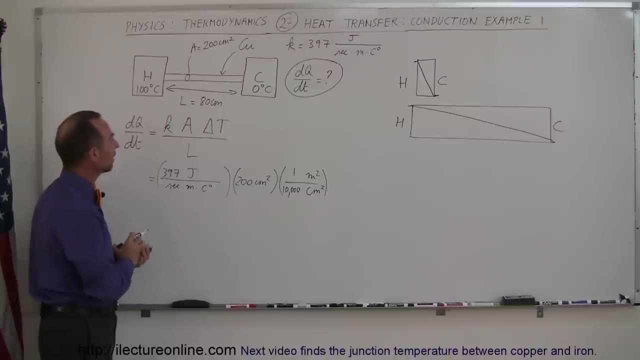 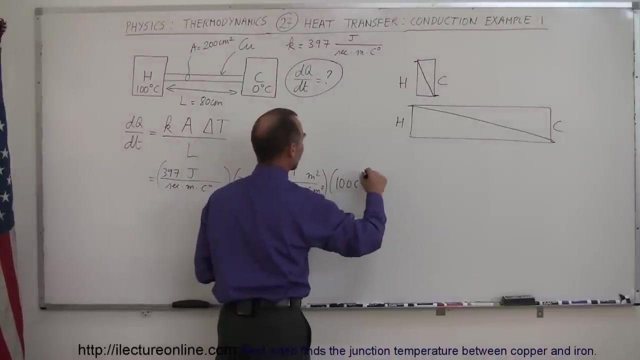 So we have a meter squared, centimeters squared, and one square meter is 10,000 square centimeters. so we add that up. We have a good conversion there. The next is the difference in the temperature. Well, the difference between 100 and 0 is 100, so that's times 100 centigrade degrees. 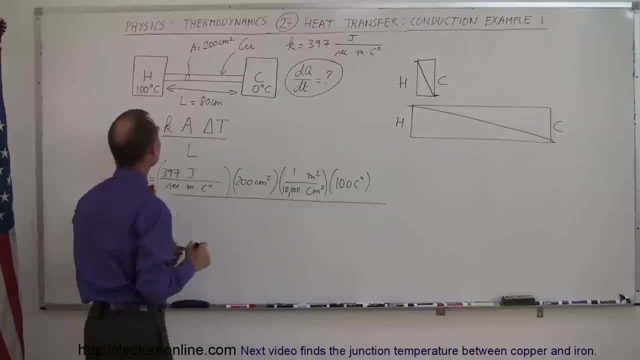 and we divide the whole thing by the length of the path, 80 centimeters is 0.8 meters. Okay, now let's see if we can cancel some things out. So square centimeters, we get rid of that Centigrade degrees that cancels out. 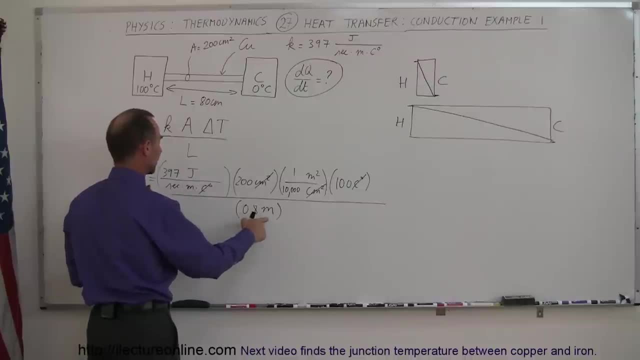 Per meter and meters. Hmm, that would be meters squared. Let's see here, That would go in here and that counts out the meters squared there. So this one counts out those two meters and we're left with joules per second. 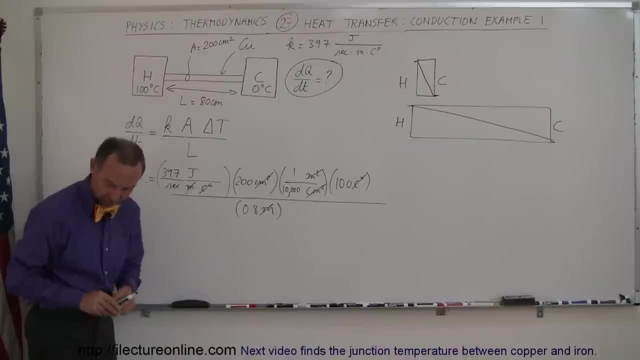 That's energy per unit time, So those are good units. So I need my calculator. Here it is, and let's find out what the amount of heat transfer is per unit time, So 397 times 200 divided by 10,000.. 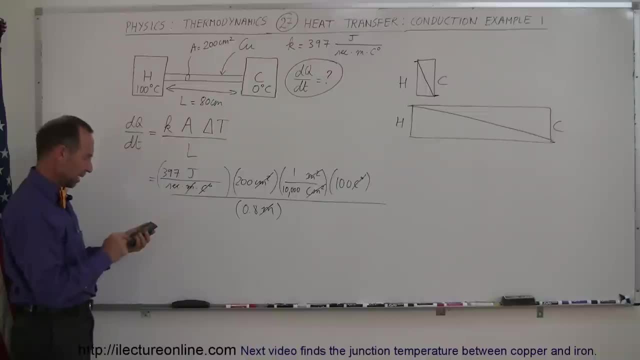 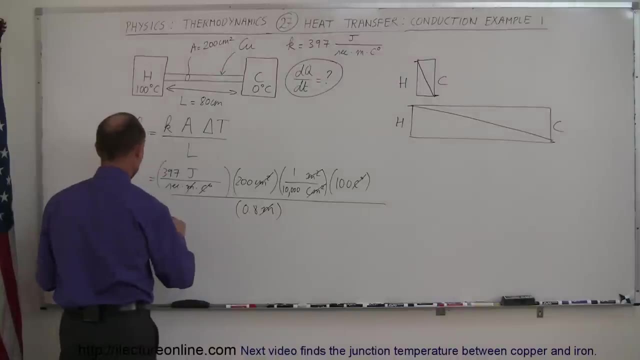 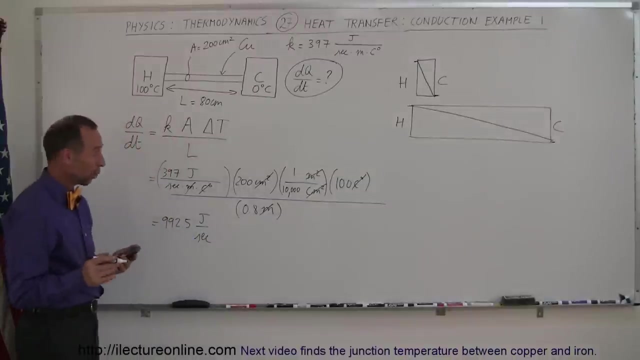 Multiply times 100.. Divide by 0.8.. Equals, and what do we get here? 992.5,, so that's equal to 992.5 joules per second, And of course joules per second is watts, and so we can then convert that to about 1,000 watts. 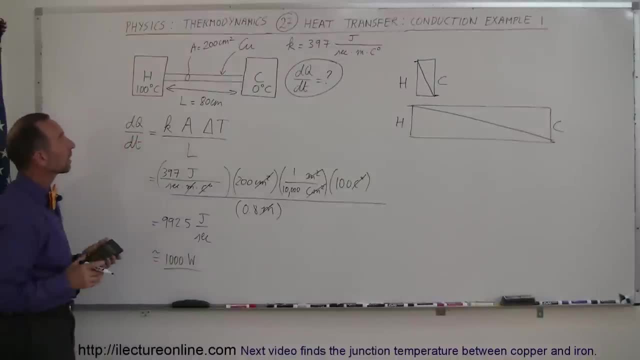 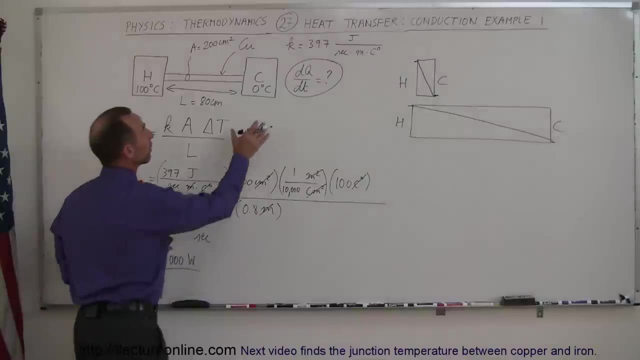 So almost 1,000 joules per second will travel along that copper bar if one side is kept at 100 degrees centigrade and the other side is kept at 0 degrees centigrade. Of course, to do that, we probably want to pack this in an ice bath. 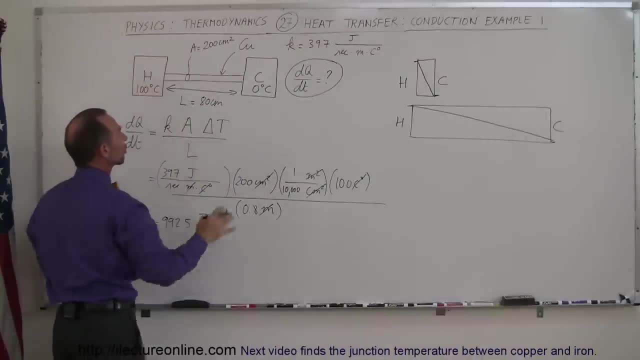 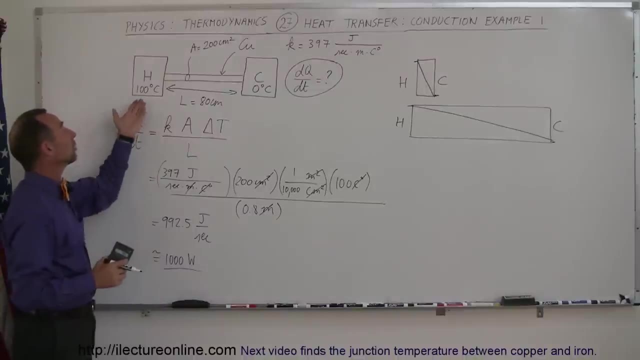 and we probably want to pack this in boiling water to keep that temperature constant, so that the heat transfer will be constant, like that. A more difficult problem would be, of course, is, let's say, we don't keep these objects at a constant temperature.